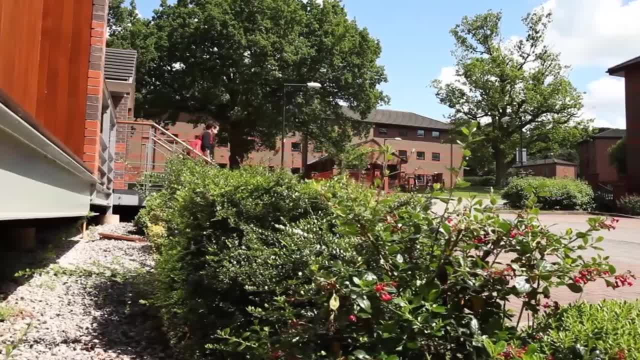 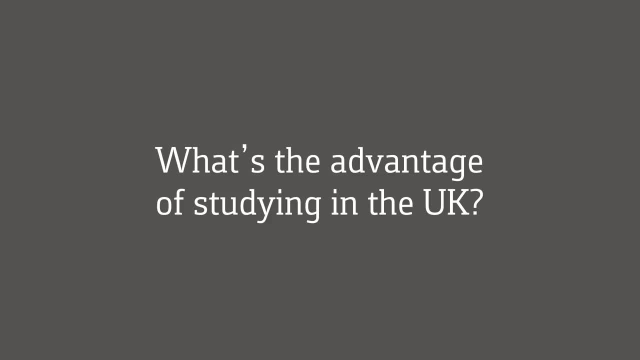 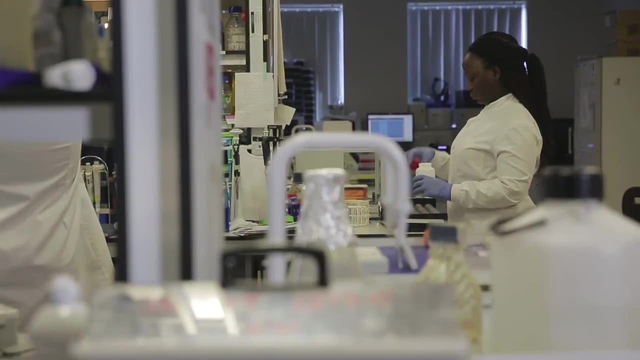 good nature, It's beautiful. The campus is really, really beautiful. So those are my first impressions and I'm like, yeah, UK. Yeah, the advantage is, you know, I've got better experience and being in KU has helped. 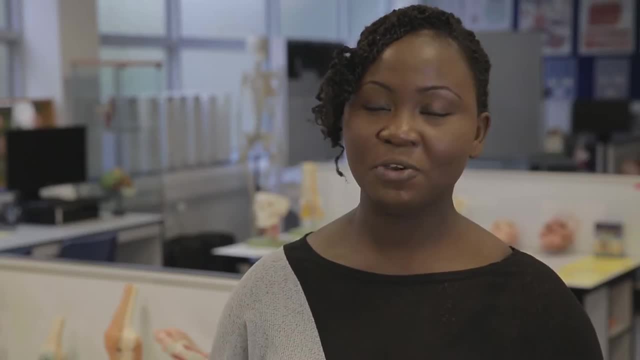 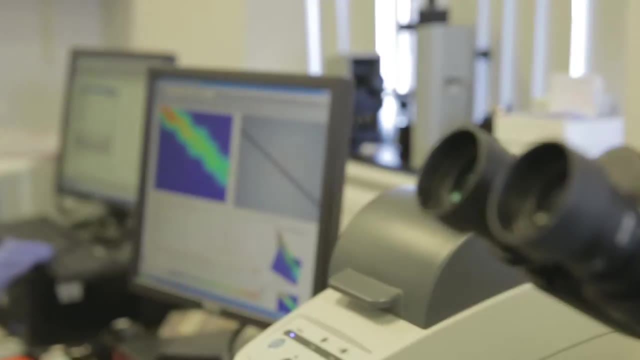 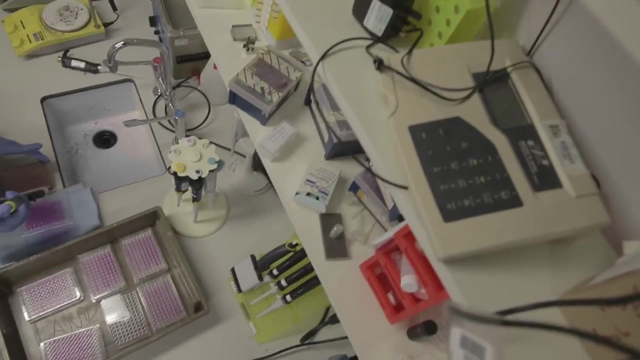 achieve all of these because I'm not just being taught theoretically. I could see what I'm being taught and it's kind of it has helped me And I've learned and get more knowledge. Yeah, I'm going to go back to Nigeria after my course and get a job and I'm really, really confident. 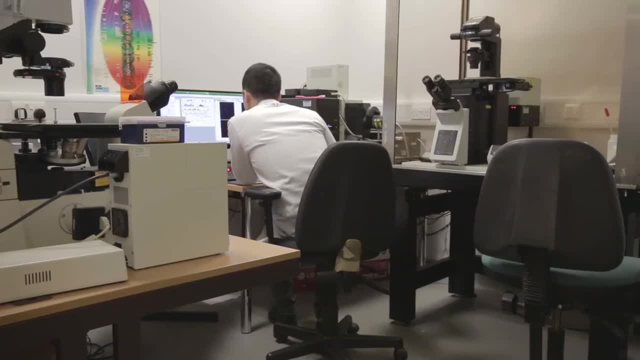 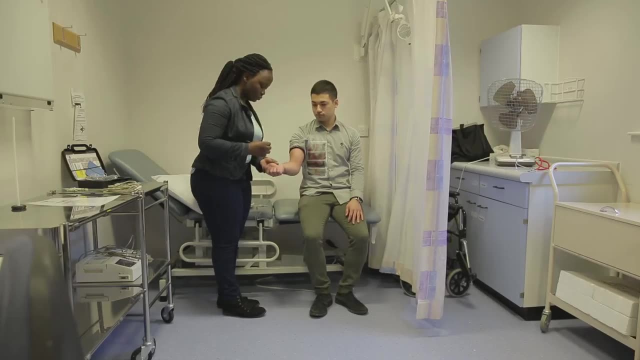 about it because my course is accredited and I feel so confident that I already have the basics of everything I need to know in that field. So I'm really, really confident of getting a good job back home. I'm actually thinking of going to the, you know, health sector, the maintenance part. 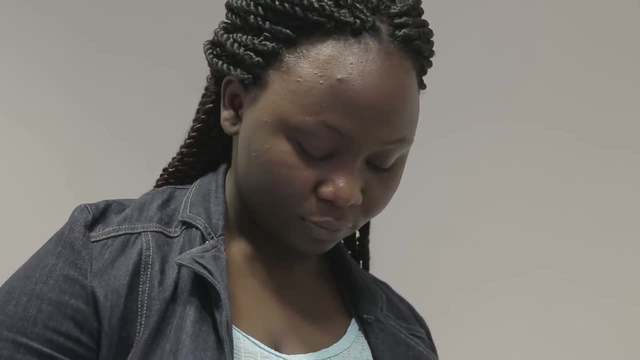 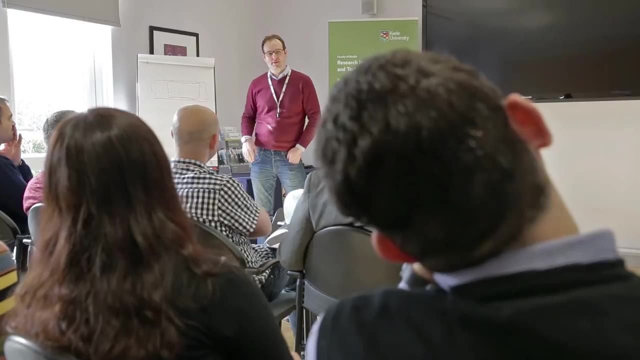 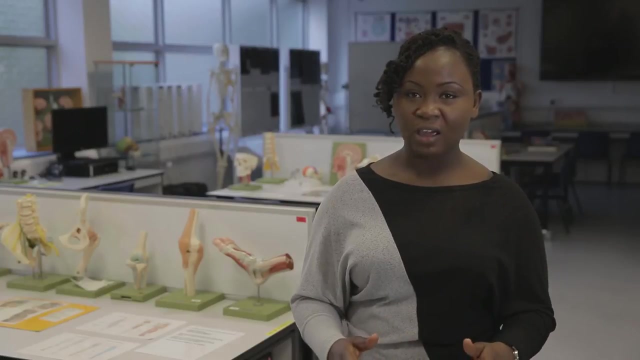 of it and all of that, or in the industries. They're really, really supportive and it just depends on you going to ask the right question, and it's not only in the academic aspect. They ask about your accommodation: are you settling in? and you've got personal tutors as well? That's something I find so. 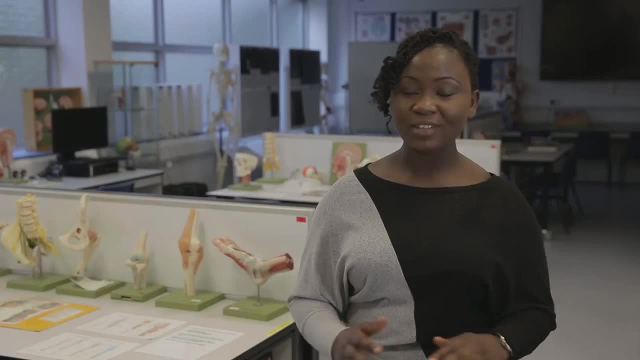 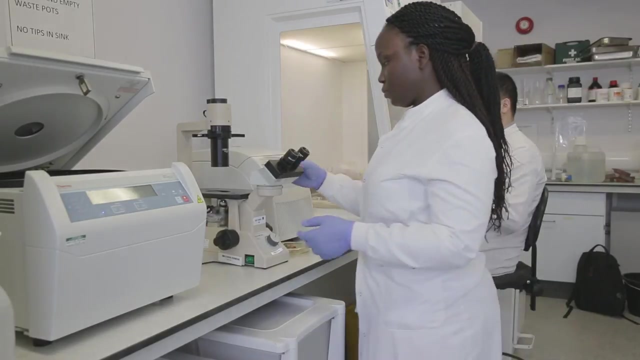 interesting and very, very helpful and, in short, they're very supportive. Life as an international student has been interesting Because you get to meet a lot of other students from other countries, and it's helpful. Even if you need English tutorials, there are English lectures to help you to you know, develop. 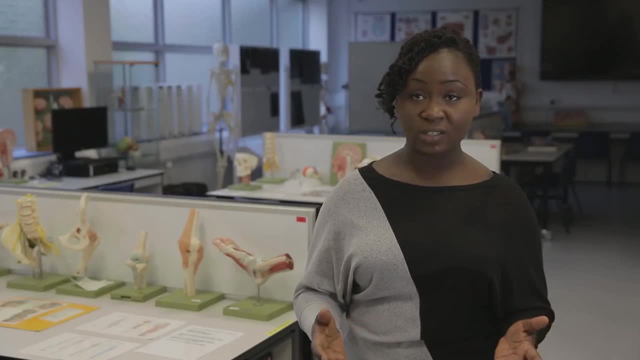 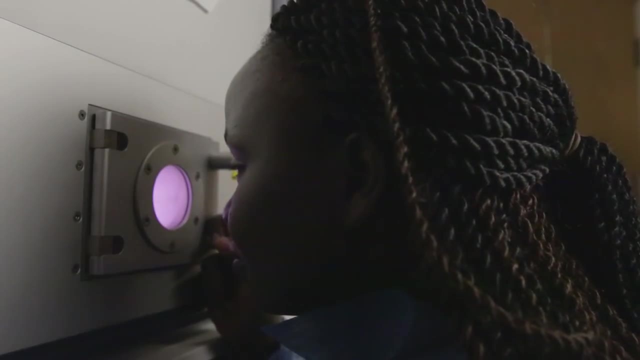 and help you with your confidence in writing, your writing skills and all of that. So it's been really helpful and it's been a supportive university for international students. It was easy to apply and you know when I first started. you know when I first started. 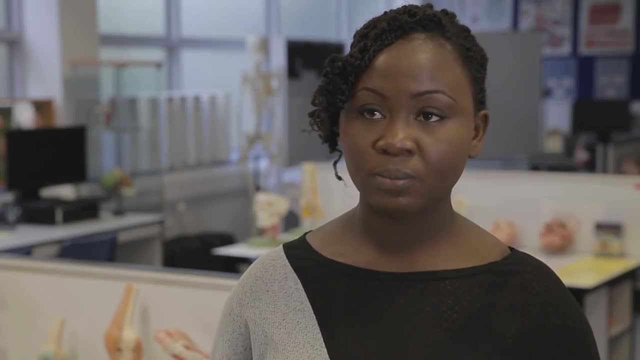 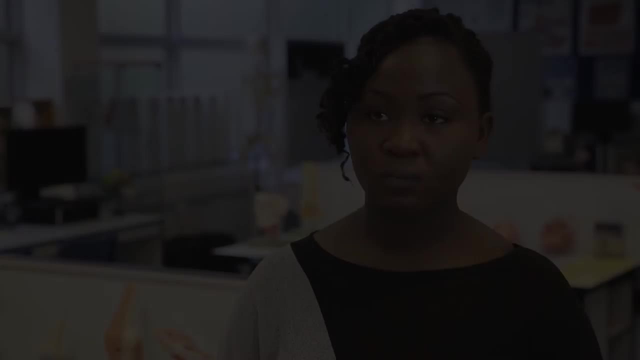 and all of that, so it was easy applying online.